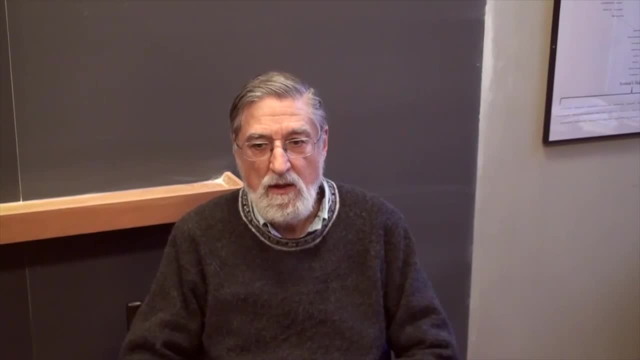 with the exact quantization of the Hall conductance. What the edge states help us to do is to see and understand, in a way somewhat complementary to Lofman's argument, why the quantization can remain exact even in the presence of impurities and electron interactions. In order to see, 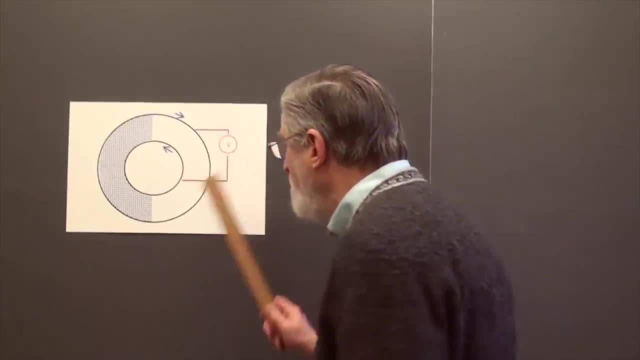 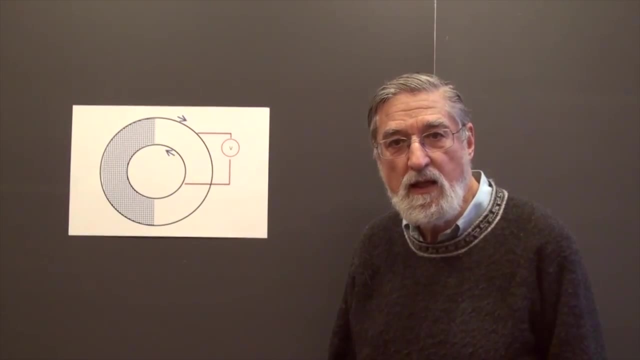 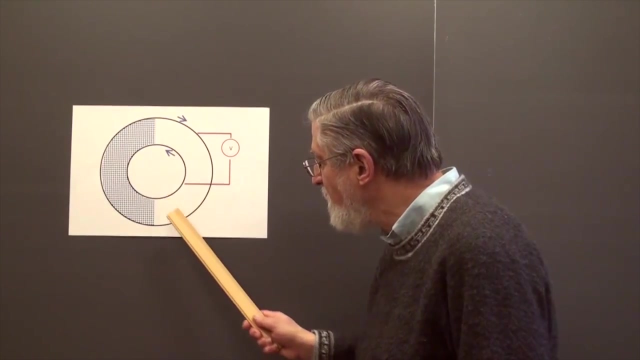 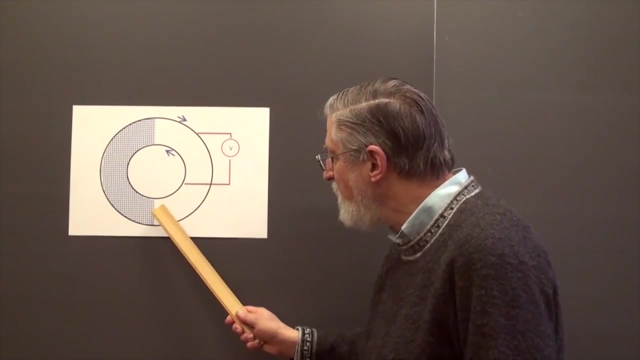 this. let me bring your attention to this figure that I have posted over here. This is supposed to represent a two-dimensional electron gas in an annular called binogeometry. This is the two-dimensional electron gas. It is bounded by these two edges and I've divided the ring into two parts. You can. 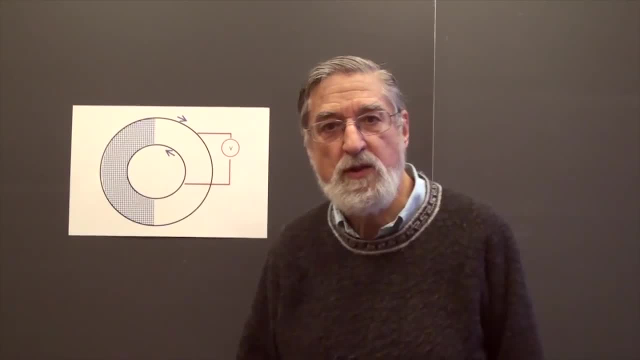 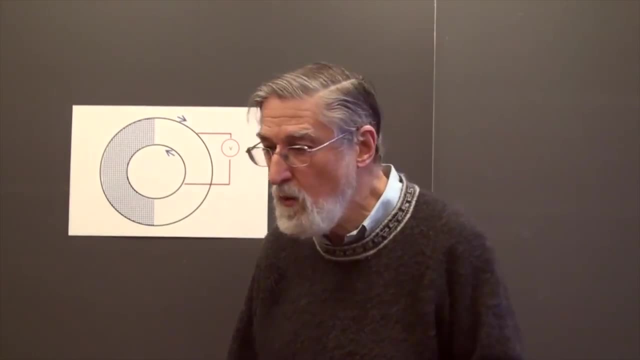 see in this part, the white region is supposed to be a region where there are no impurities and the electron-electron interaction is turned off. So this is an ideal system and we already know what will happen if the Fermi level is in between two Landau levels There. 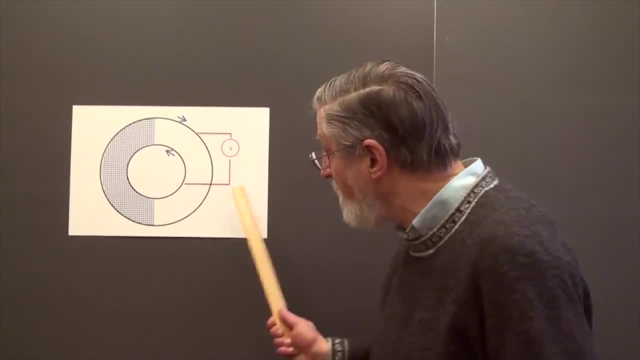 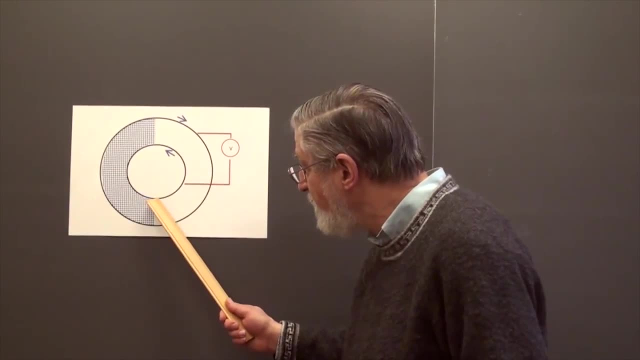 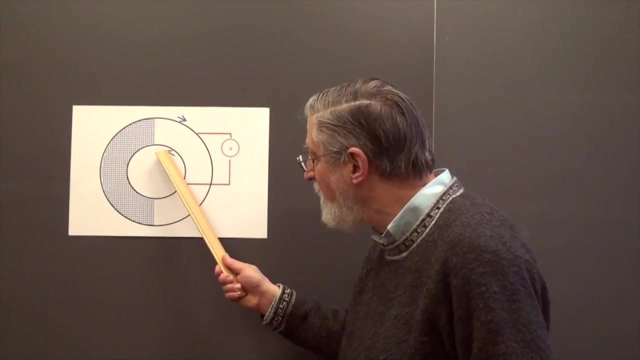 are no states in the bulk at the Fermi level, The system is not going to be able to do anything about it. This is a quantized Hall state, but there will be, of course states at the Fermi level along the edges. These will be the chiral edge states which propagate in the direction. 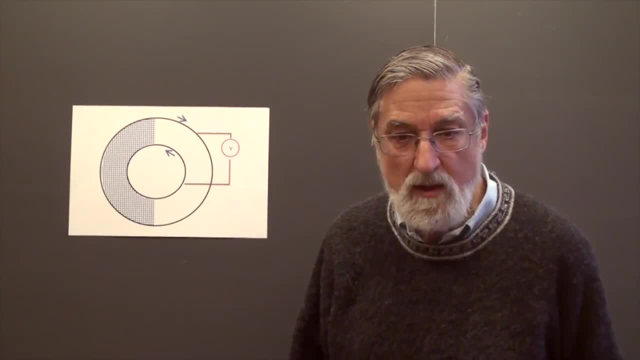 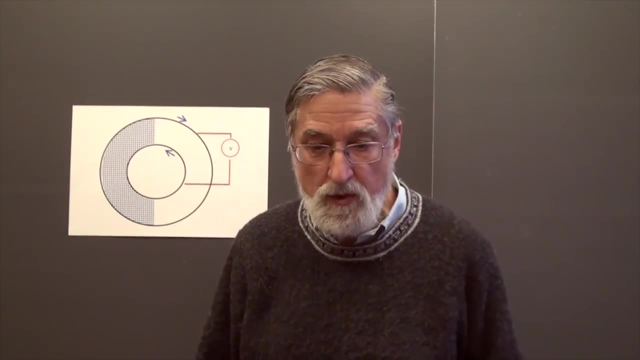 of the arrows to the opposite directions at opposite edges. Now in this region here I'm assuming that we have some impurities and perhaps also have turned on some electron-electron interaction, and we know that if we introduce impurities that can easily produce states at the Fermi level. 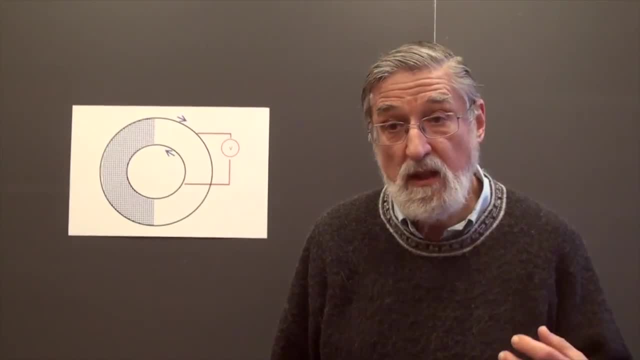 Now in this region here I'm assuming that we have some impurities and perhaps also have turned on some electron-electron interaction, and we know that if we introduce impurities that can easily produce states at the Fermi level. But these states will be tied to the impurities. and if the number of impurities is not too, 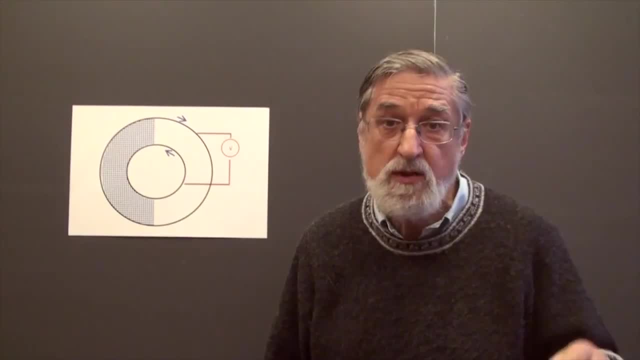 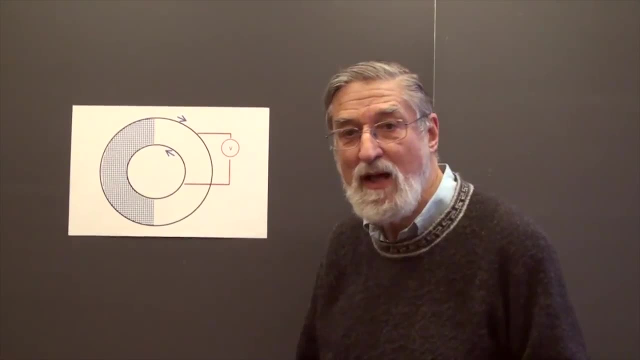 large. these states will be localized about the individual impurities with a localization length of the order of the magnetic length. And if the distance from the inner and outer, between the inner and outer edges of the samples, is very large compared to this localization length, it is very difficult, very possible. 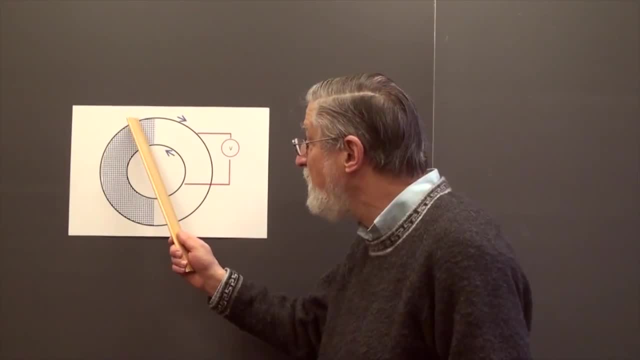 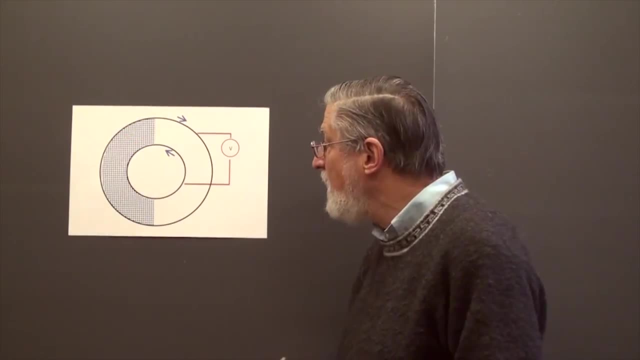 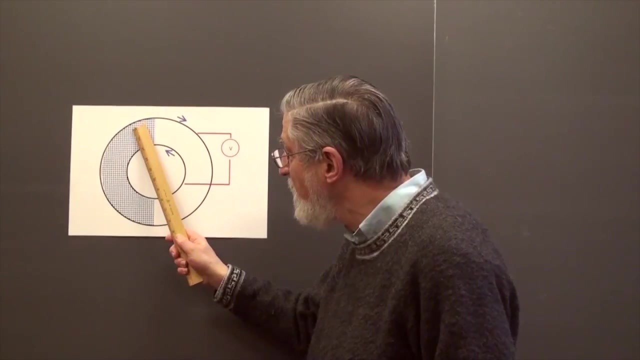 for an electron at low temperatures- zero temperature, low voltage- to get across from one edge to the other. This region is basically insulating. Okay, and that is an important factor. The other factor is that there will. well, there are no. there are only localized states. 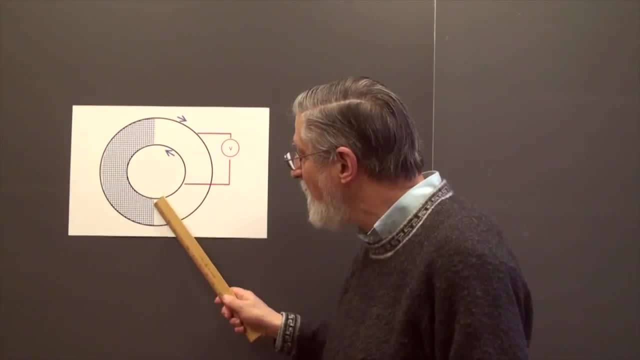 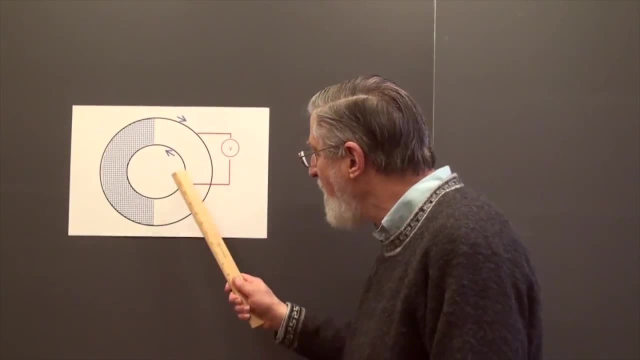 at the Fermi level in the bulk. There still have to be extended states around the edges, as we shall see, in order to carry current. Okay, so now we can imagine what happens if we add a bunch of electrons in this inner edge here. 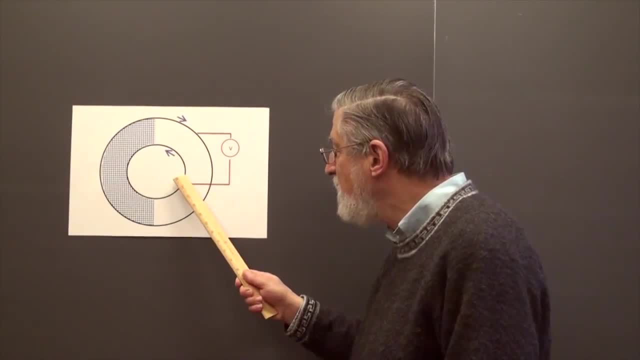 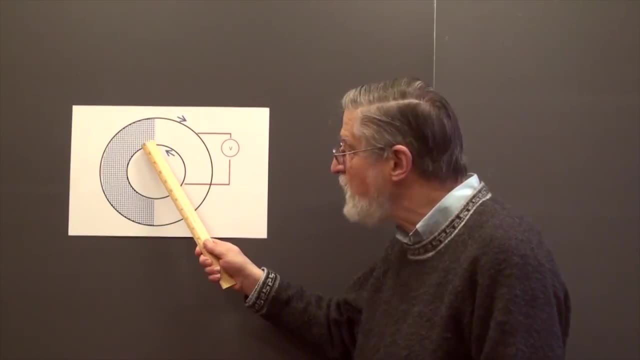 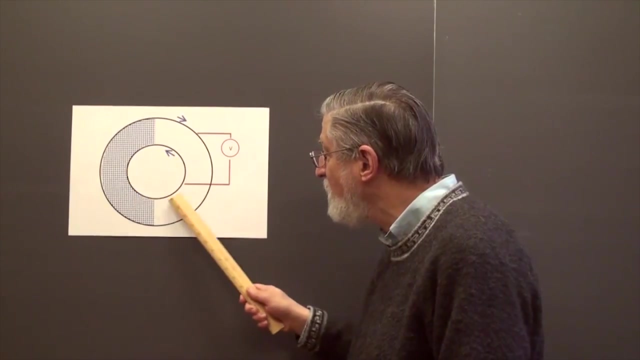 Let's say at this point here and ask what happens. It will, of course these electrons will propagate in the direction of the arrow around the edge until they get to this shaded area where they have to still continue because current has to be conserved, and they will keep going around and around, but they will stay on this. 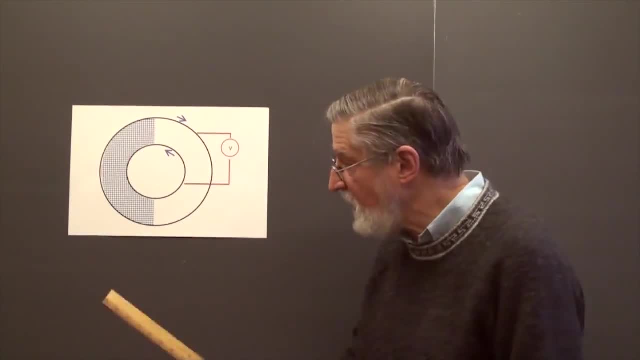 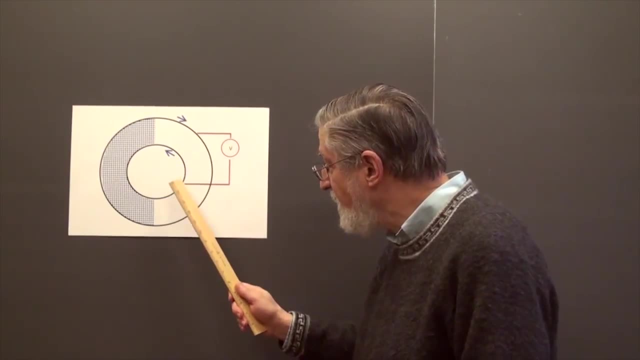 edge, because they can't tunnel from the inner edge to the outer edge at low temperatures. So eventually they will reach some kind of thermal equilibrium state where they will be able to move around, And then we can define a chemical potential or more precisely, an electrochemical potential. 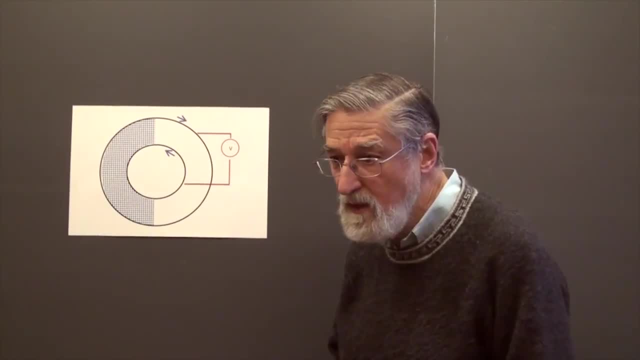 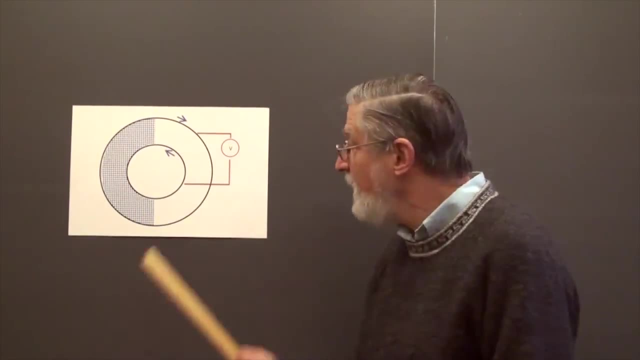 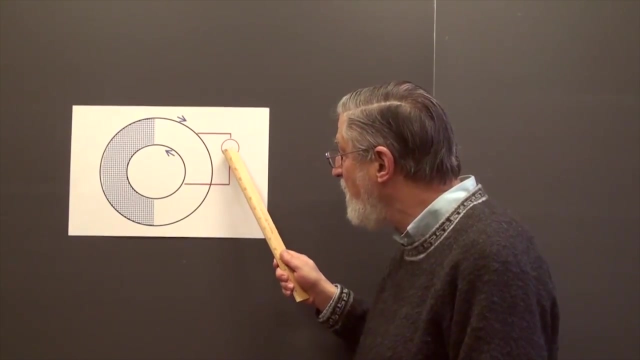 which has to be a constant all the way around this edge and can be different from the electrochemical potential defined on the outer edge. If we connect a voltmeter between the inside edge and the outside edge, the voltmeter- the Idle voltmeter- will exactly measure this difference in electrochemical potentials. 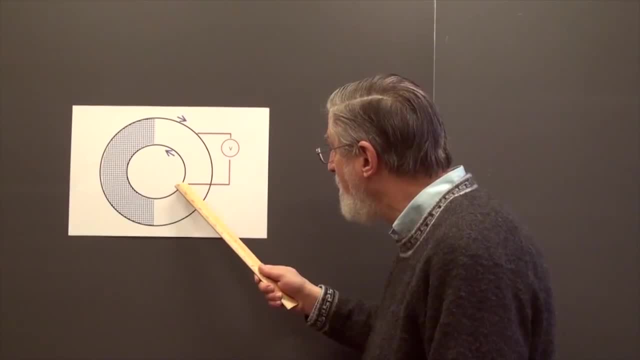 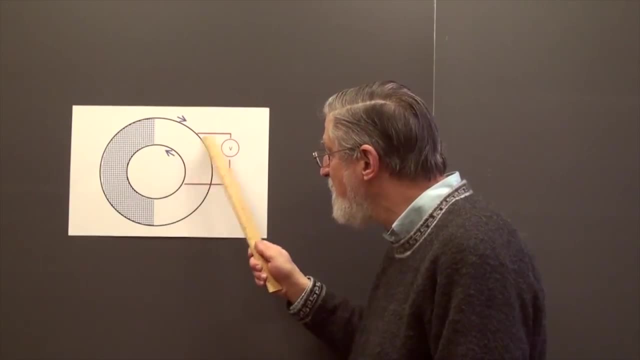 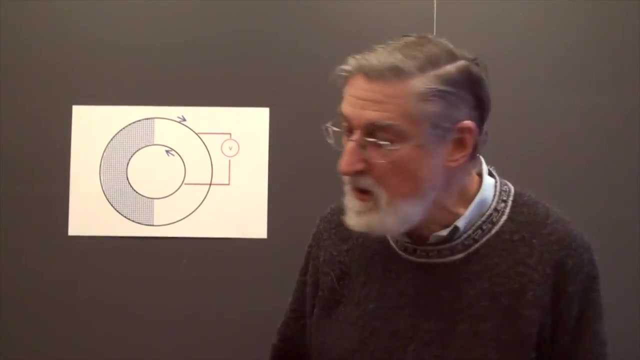 Okay, And if it draws no current, then this can continue forever. If it draws a small amount of current, we can add a battery to maintain that current and keep these two edges at different voltages independent of time. Now we can ask what happens to the current? 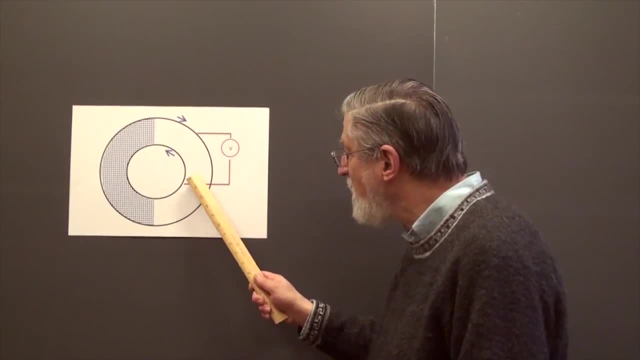 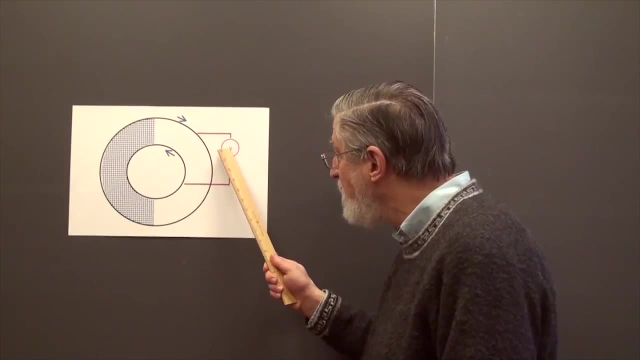 We know that in this region, which is an ideal quantized Hall conductor, there will be a current, a net current, flowing in, say, in this direction, which will be equal to the voltage times, the quantized Hall conductor. What happens when this current gets to this edge? 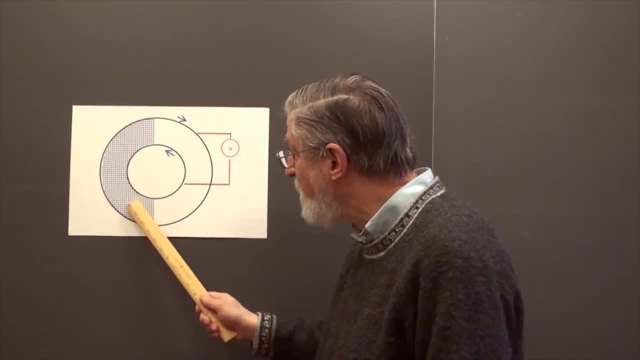 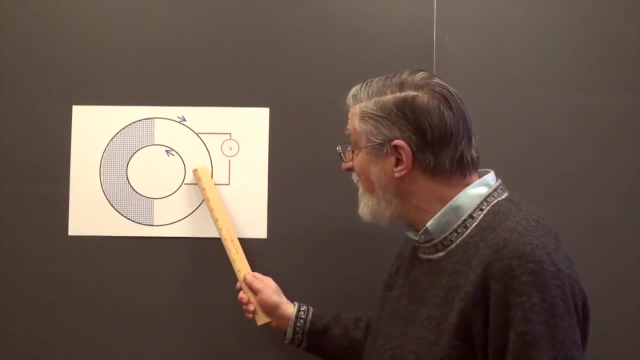 Well, if we this part of the sample, if we, if we're in equilibrium and then we're in a steady state, we know that charge has to be conserved. so therefore, the current cannot have any divergence and the current must be the same everywhere around this loop. 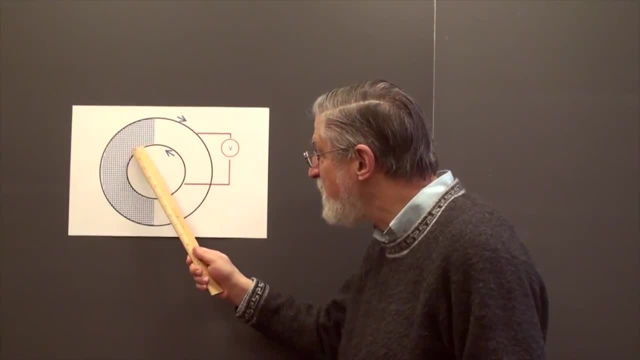 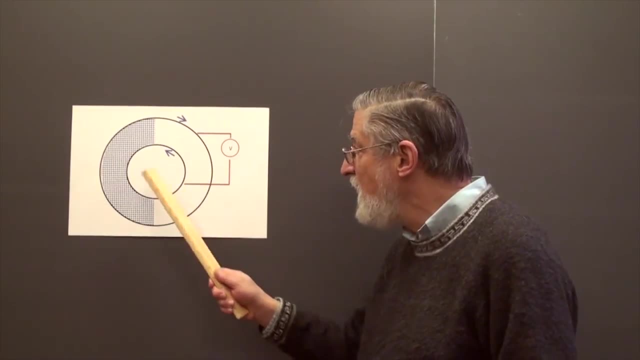 Well, we also know that the voltage we've reached equilibrium, so the voltage is constant on this edge and this edge The voltage difference between these two points is the same as the voltage difference between these two points. And the current is the same, so the current is still related to the voltage difference. 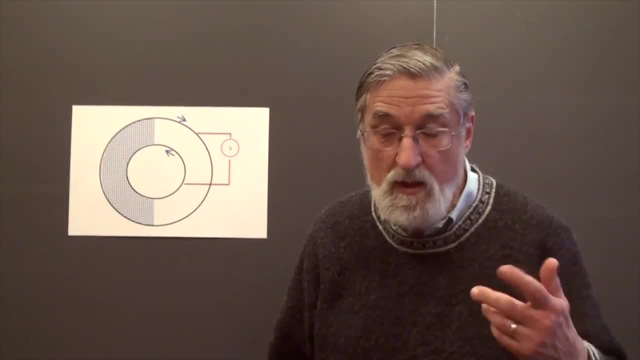 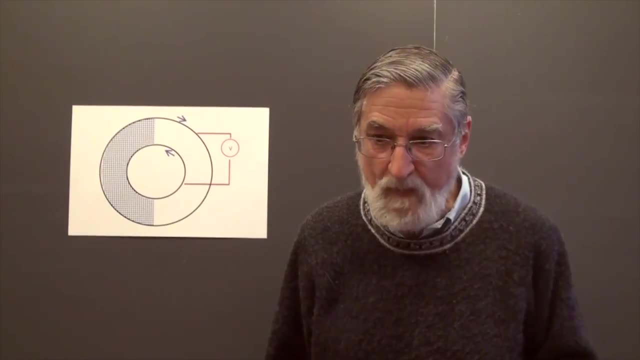 by precisely the same ratio, namely the quantized Hall conductance in the region where we have impurities as in the region where we don't have impurities. Now, there's something else I would like to add, though, about the role of electro-electric. 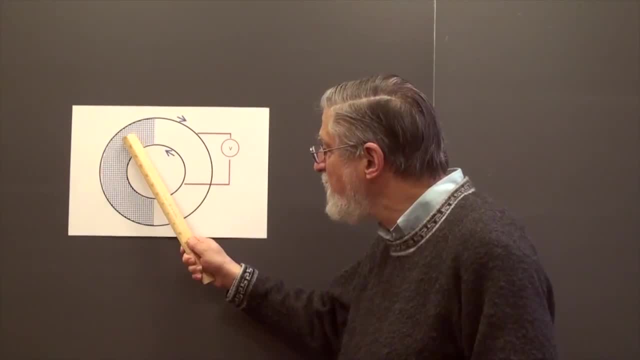 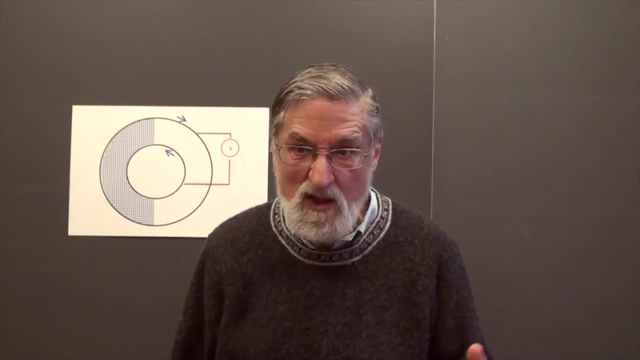 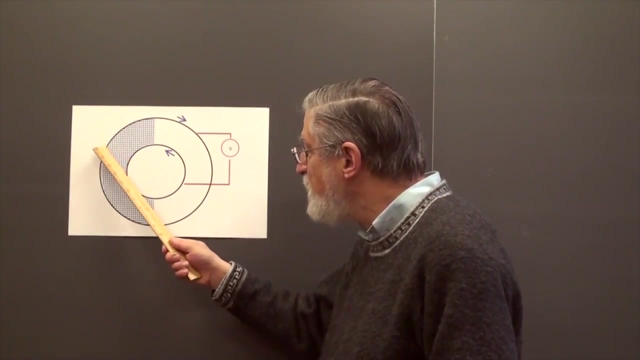 interactions, which is sometimes ignored. In this region, where we have electro-electric interactions, it is no longer true that the current is entirely carried by the edge states. If you have electro-electric interactions and we have a different charge density on the two edges, there will in general be an electric field pointing from, say, the outer. 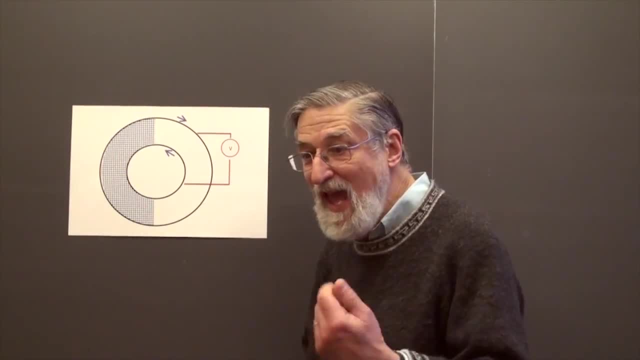 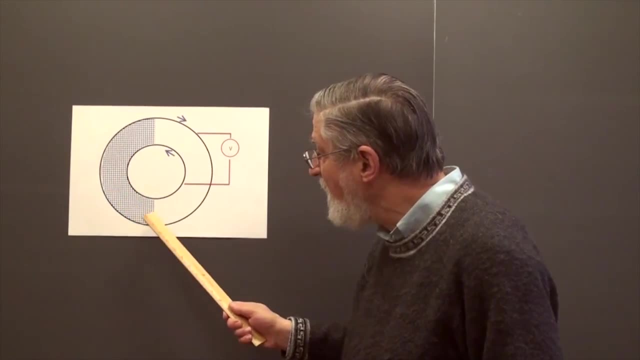 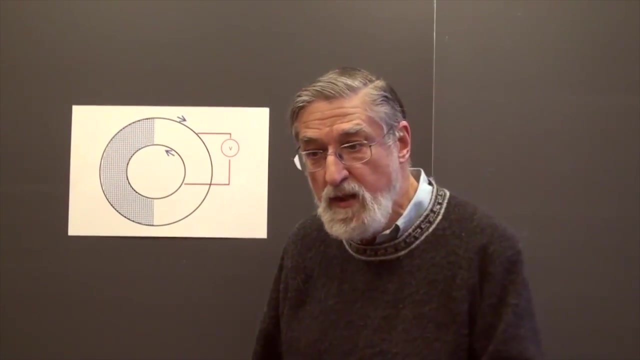 edge to the inner edge and that electric field can drive a bulk current in the bulk in this system, even though the states at this Fermi surface are completely local on the Fermi surface, We know that there'll have to be states below the Fermi energy, in the middle of lambda levels. 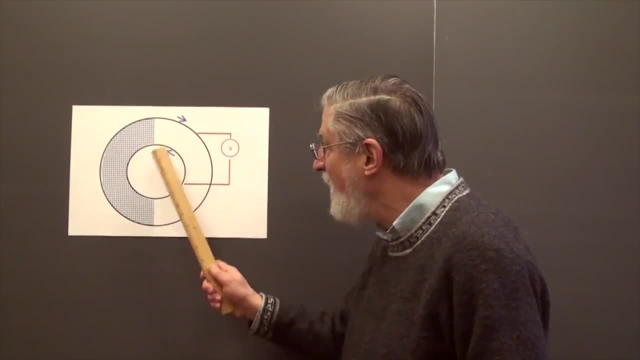 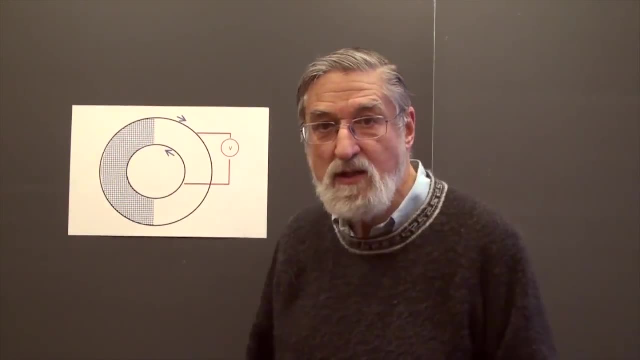 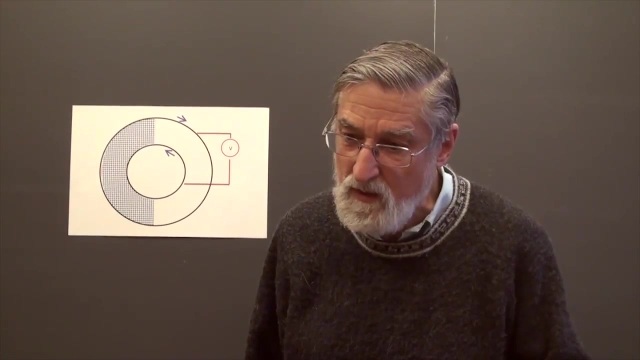 which are delocalized and can extend around the sample and it's perfectly allowed for an electric field to produce a current flowing around these states below the Fermi surface that we cannot have a current flowing parallel to the electric field in the state below the 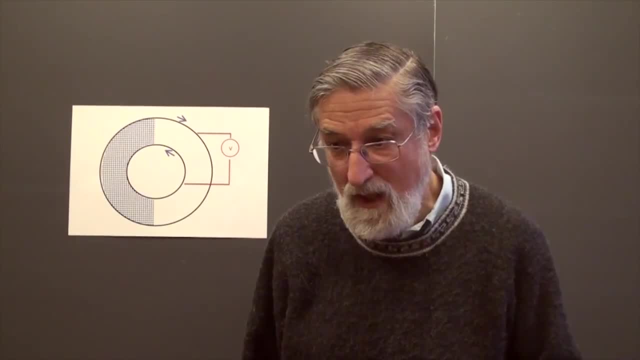 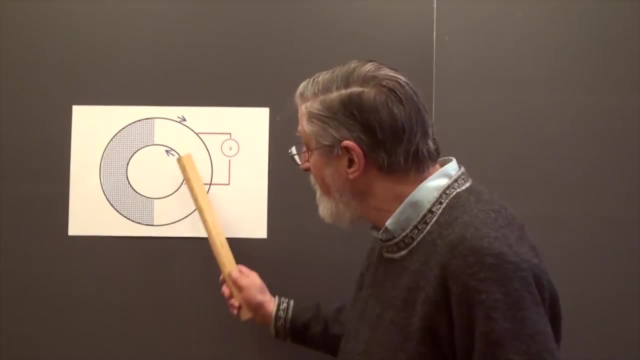 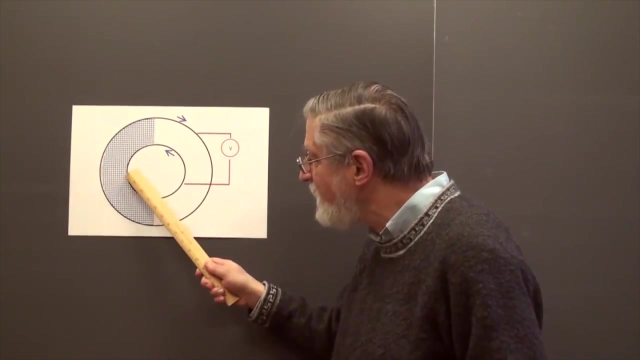 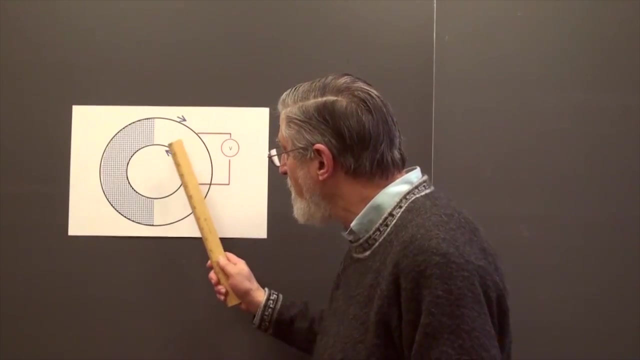 Fermi surface. That's why, essentially, charge conservation and current charge and energy conservation. but we can have current flowing parallel to the electric field. we can have current flowing perpendicular to the electric field and that's what happens. So in the case where there are electro-electric interactions, the current is not confined.